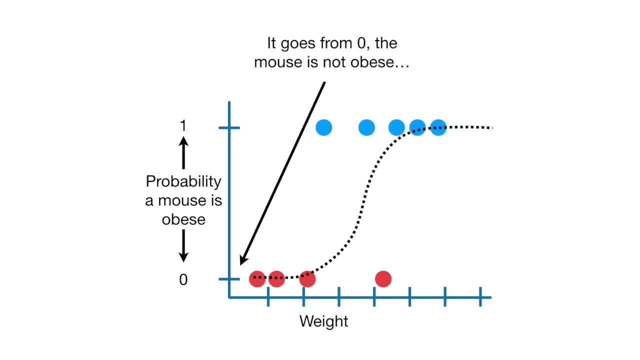 is obese. It goes from zero- the mouse is not obese- to one the mouse is obese. The dotted line is fit to the data to predict the probability a mouse is obese given its weight. If we weight a heavyweight mouse then the corresponding point on the line indicates: 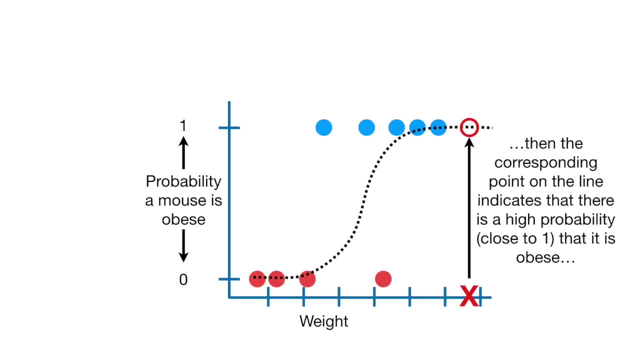 that there is a high probability- close to 1, that it is obese. And if we weight a middleweight mouse, then there is an intermediate probability- close to 0.5, that it is obese. Lastly, a lightweight mouse has a low probability- close to 0, of being obese. 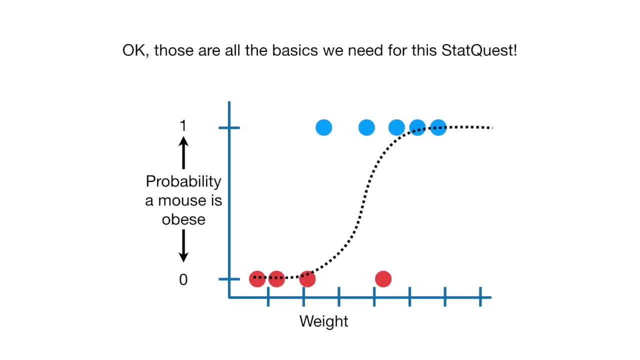 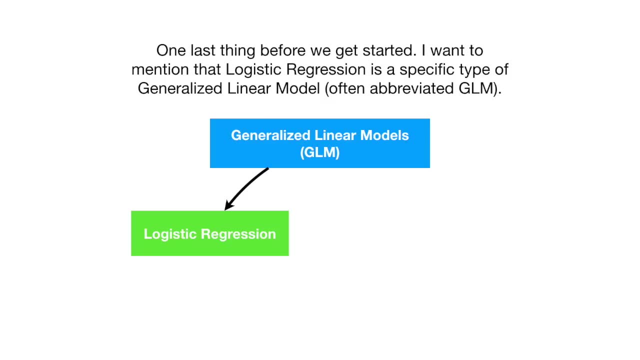 Okay, those are all the basics we need for this stat quest. One last thing before we get started. I want to mention that logistic regression is a specific type of generalized linear model, often abbreviated GLM. Generalized linear models are a generalization of the concepts and abilities of regular linear 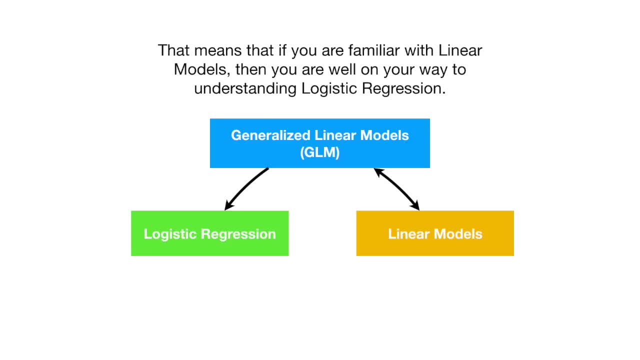 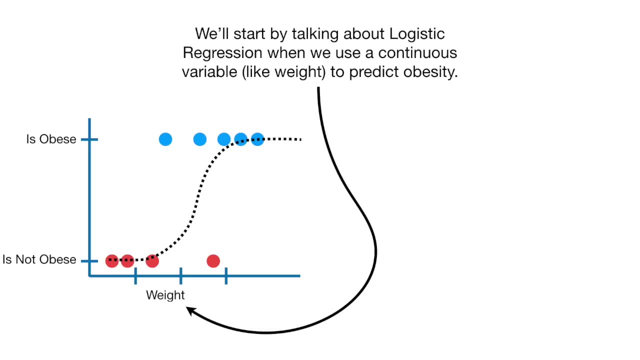 models, which we've already talked about in many stat quests. That means that if you're familiar with linear models, then you're well on your way to understanding logistic regression. We'll start with the first example. We'll start by talking about logistic regression when we use a continuous variable like weight. 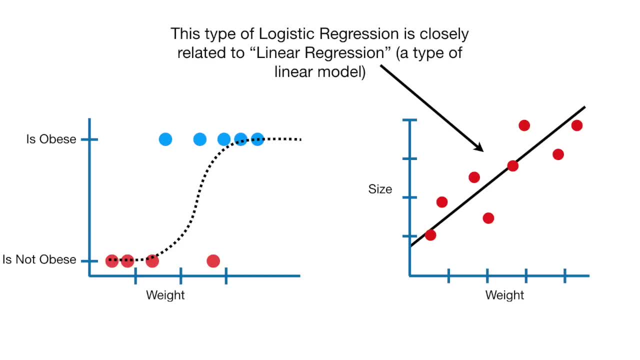 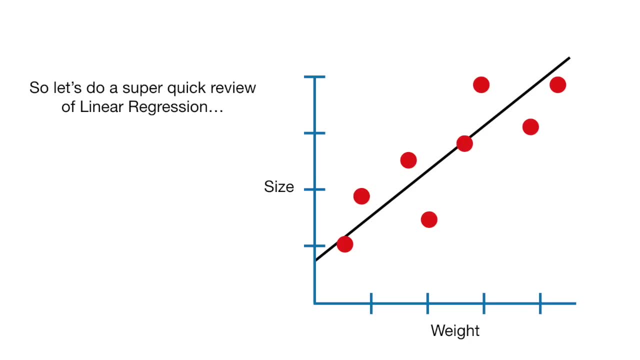 to predict obesity. This type of logistic regression is closely related to linear regression, a type of linear model. So let's do a super quick review of linear regression- Shameless self-promotion. If you're not already familiar with linear regression, check out the stat quests on linear. 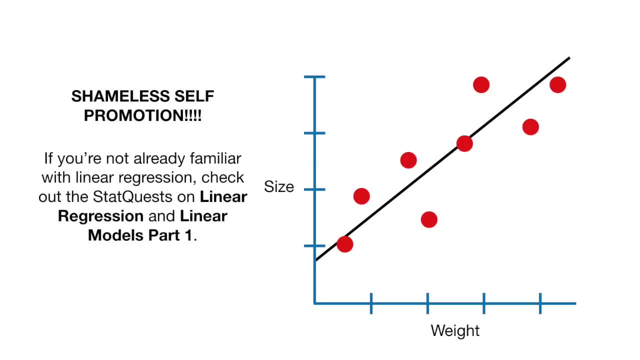 regression and linear models. part 1.. OK, we start with some data And we fit a line to it And this is the equation for the line: It has a y-axis intercept and a slope And we plug in values for weight to get predicted values for size. 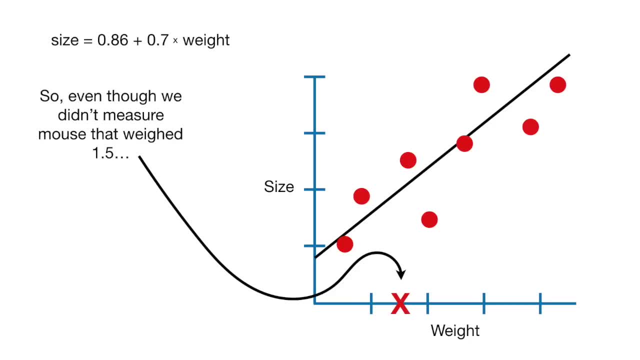 So, even though we didn't measure a mouse that weighed 1.5,, we can plug 1.5 into the equation And predict that mouse to have size 1.91.. And a mouse with weight 1.5 and size 1.91 would end up on the line at this point. 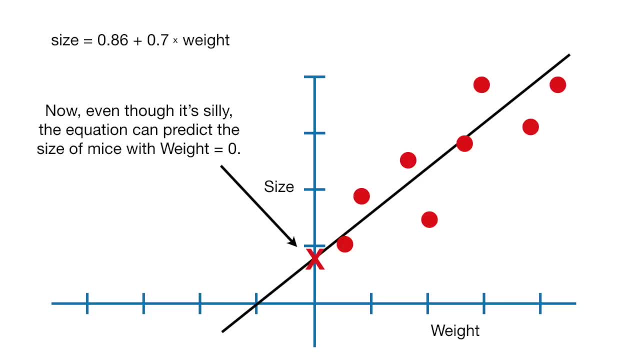 Now, even though it's silly, the equation can predict the size of mice with weight equals zero. That's just the y-axis intercept 0.86.. And we can even predict the size of mice with weight equals zero. I'm pointing this out because the fact that we are not limiting the equation to a specific 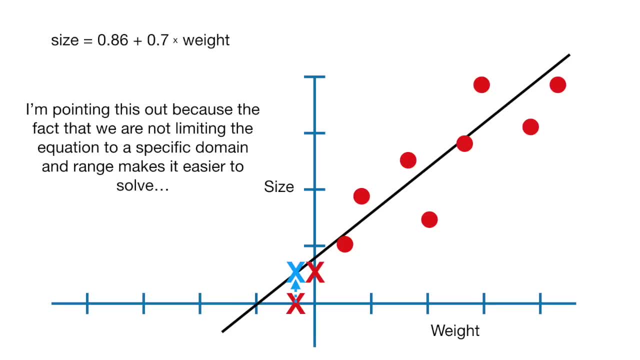 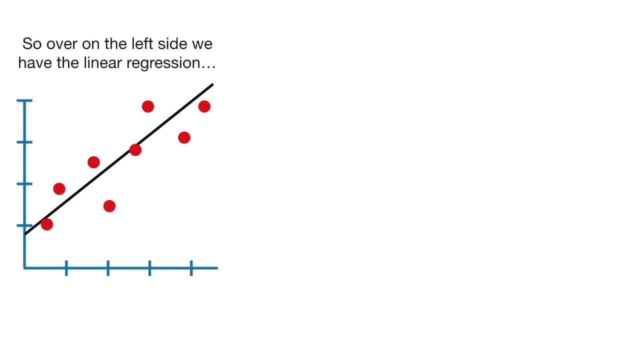 domain and range makes it easier to solve And this has a big effect on how logistic regression is done. So over on the left side we have the linear regression And on the right side we have the logistic regression. With linear regression the values on the y-axis are the same. 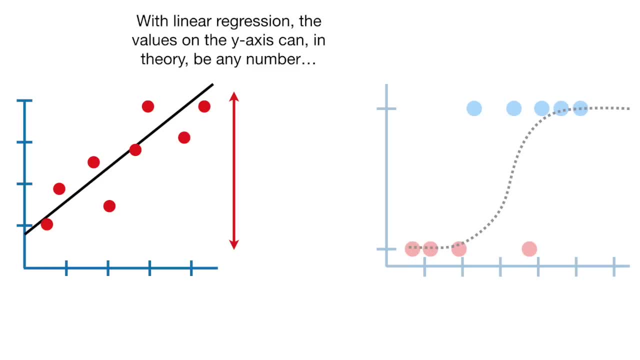 So we have the linear regression And on the right side we have the logistic regression, And on the left side we have the logistic regression. The y-axis can in theory be any number. Unfortunately, with logistic regression the y-axis is confined to probability values between. 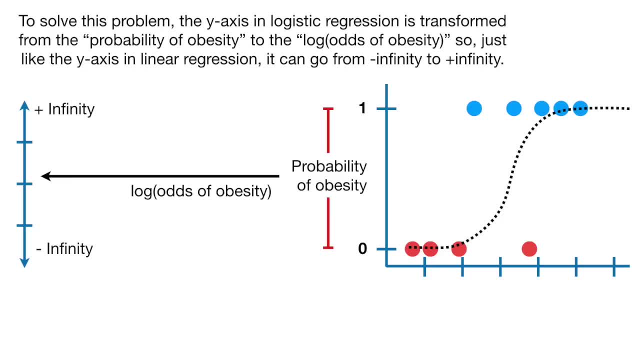 0 and 1.. To solve this problem, the y-axis in logistic regression is transformed from the probability of obesity to the log odds of obesity. So, just like the y-axis in linear regression, it can go from negative infinity to positive infinity. 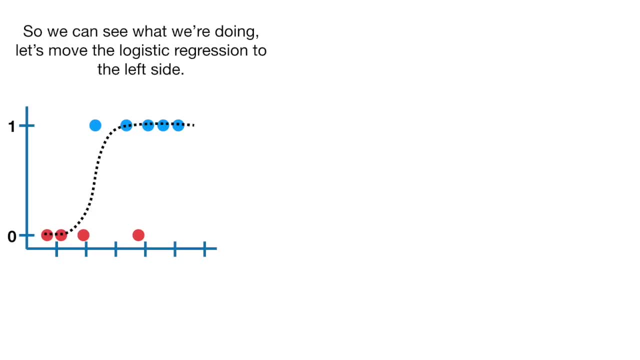 So we can see what we're doing. let's move the logistic regression to the left side. Now. let's transform the y-axis from a probability of obesity scale to a log odds of obesity scale. We do that with the legit function that we talked about in the odds slash: log odds stat. 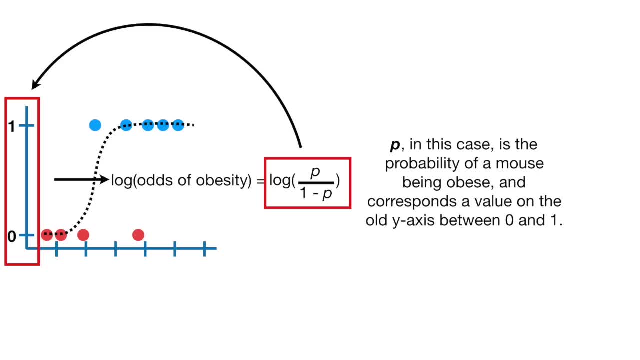 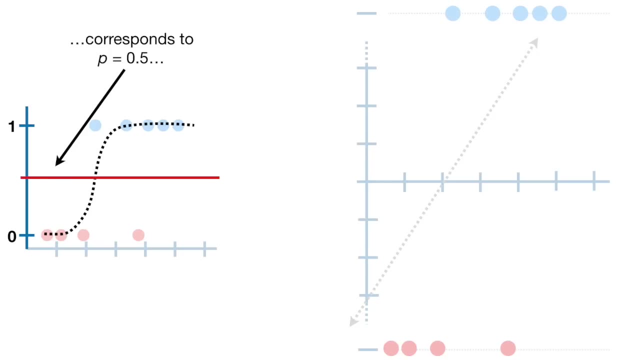 quest. P in this case is the probability of a mouse being obese and corresponds to a value on the old y-axis. The midpoint on the old y-axis corresponds to P equals 0.5.. And when we plug P equals 0.5 into the legit formula and do the math, we get 0, the center. 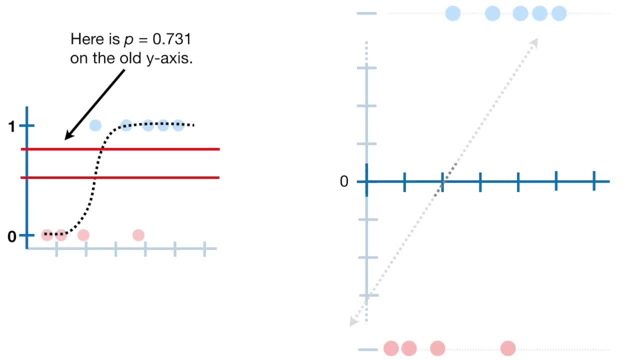 of the new y-axis. Here is P equals 0.731 on the old y-axis. If we plug P equals 0.5 into the legit formula and do the math, we get 0, the center of the new y-axis. 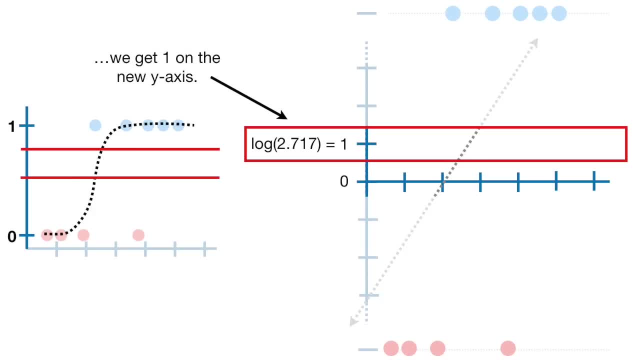 P equals 0.731 into the legit function and do the math: we get 1 on the new y-axis. If we plug P equals 0.88 into the legit function and do the math, we get 2 on the new y-axis. 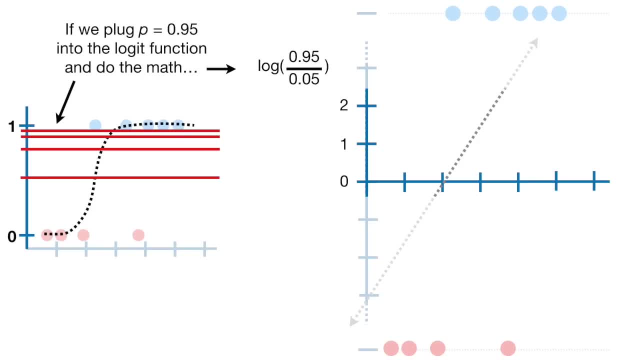 If we plug P equals 0.95 into the legit function and do the math, we get 3 on the new y-axis. Lastly, we plug P equals 1 on the new y-axis. All right, We're good to go. 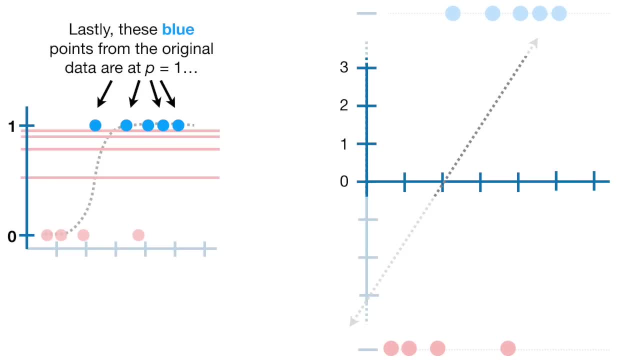 Thanks, Bye, Bye, See you in the future. Take care, drives Bye, Bye. Technically, these blue points from the original data are at p equals 1.. If we plug p equals 1 into the legit function and do the math, well, technically you can't. 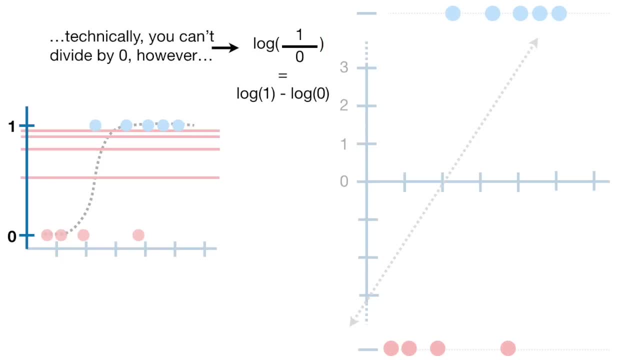 divide by 0,. however, the log of 1 divided by 0 equals the log of 1 minus the log of 0, and the log of 0 is defined as negative infinity. And since something minus negative infinity equals positive infinity, this whole thing. 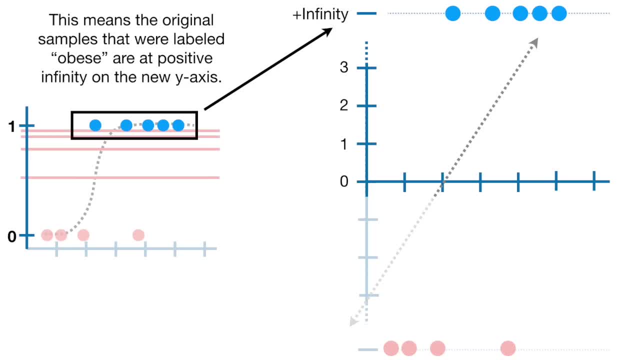 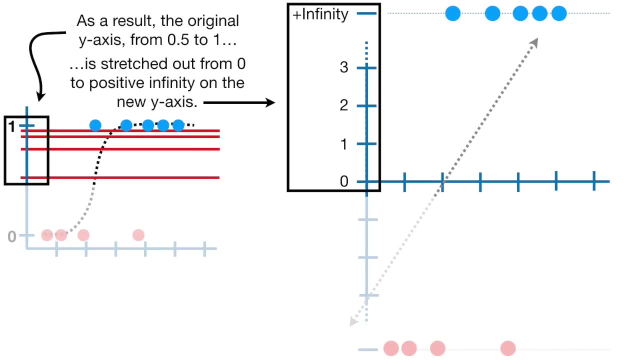 is equal to positive infinity. This means the original samples that were labeled obese are at positive infinity on the new y-axis. As a result, the original y-axis from 0.5 to 1 is stretched out from 0 to positive infinity on the new y-axis. 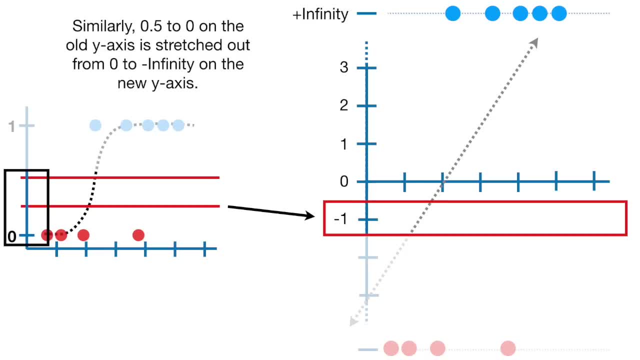 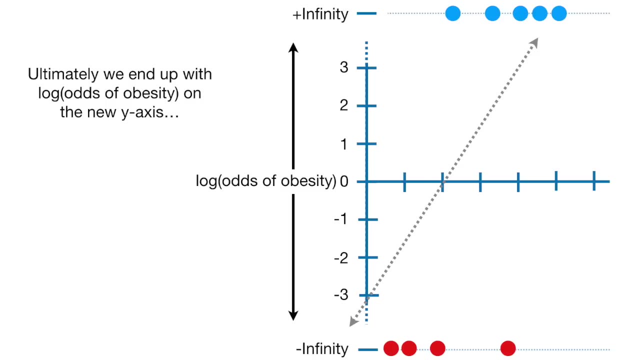 Similarly, 0.5 to 0 on the old y-axis is stretched out from 0 to negative infinity on the new y-axis. Ultimately, we end up with the log of the odds of obesity on the new y-axis, And the new y-axis transforms the squiggly line into a straight line. 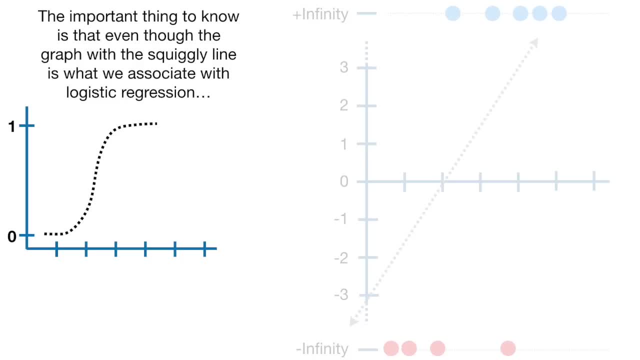 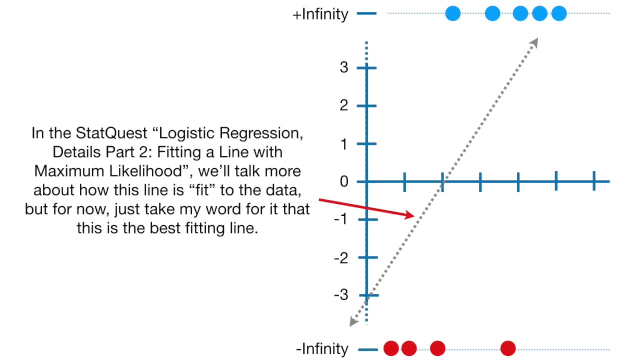 The important thing to know is that, even though the graph with the squiggly line is what we're associating with logistic regression, the coefficients are presented in terms of the log odds graph In the StatQuest Logistic Regression Details. Part 2, Fitting a Line with Maximum Likelihood. 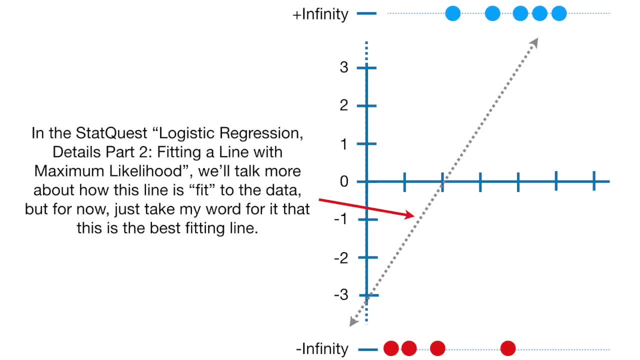 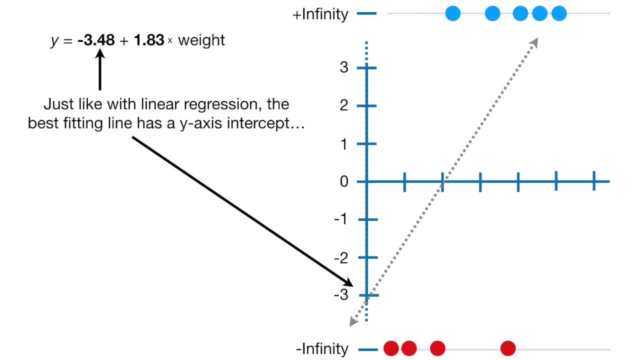 we'll talk more about how this line is fit to the data, but for now just take my word for it that this is the best fitting line. Just like with linear regression, the best fitting line has a y-axis intercept and a slope. 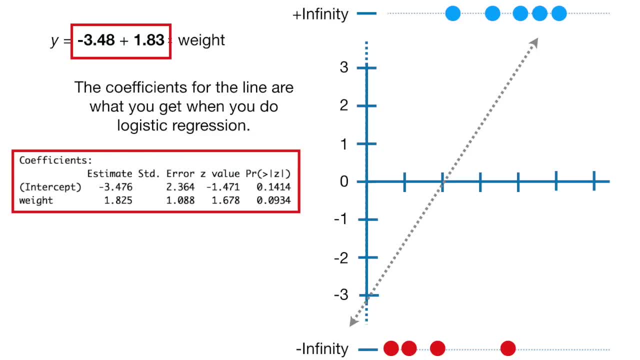 The coefficients for the line are what you get when you do logistic regression. The first coefficient is the y-axis intercept when weight equals 0. It means that when weight equals 0, the log of the odds of obesity are negative: 3.476.. 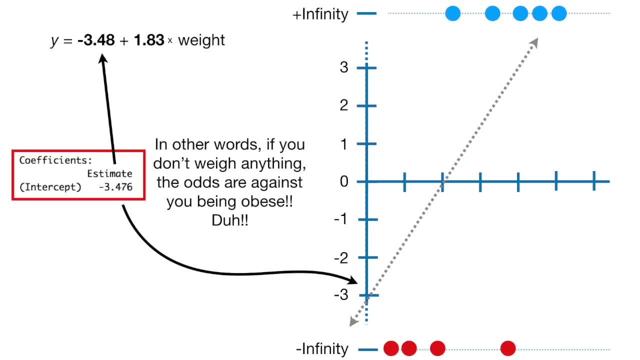 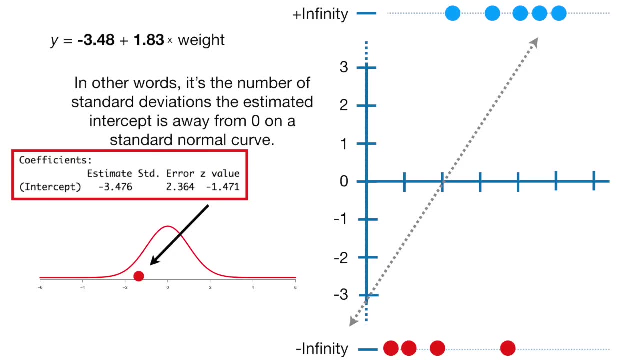 In other words, if you don't weigh anything, the odds are against you being obese. Duh, Here's the standard error for the estimated weight. The Z value is the estimated intercept divided by the standard error. In other words, it's the number of standard deviations. the estimated intercept is away. 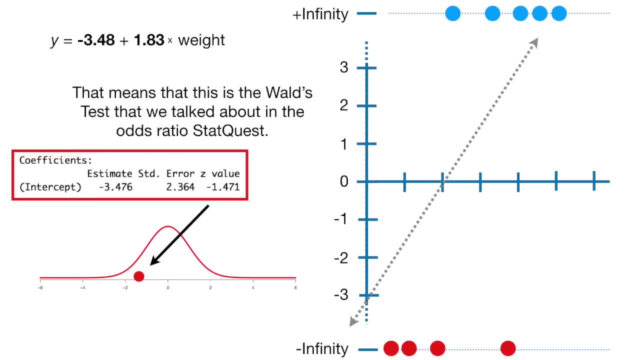 from 0 on the standard normal curve. That means that this is the Wald's test that we talked about in the odds ratio StatQuest. Since the estimate is less than 2 standard deviations away from 0, we know it is not statistically significant. 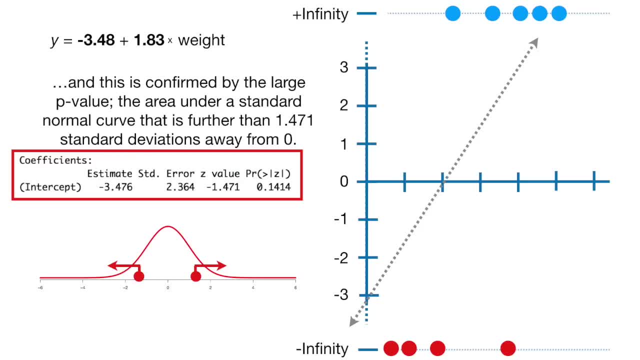 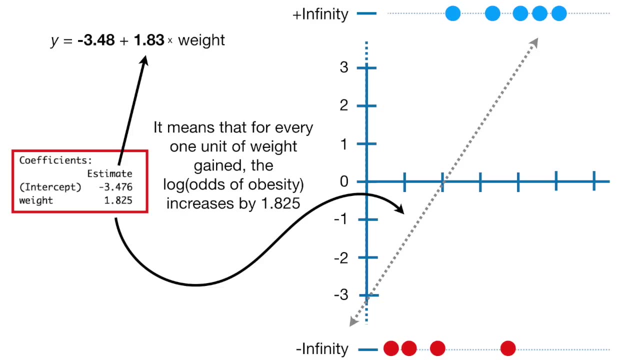 And this is confirmed by the large p-value, the area under the standard normal curve that is further than 1.47 standard deviations away from 0.. The second coefficient is the slope. It means that for every one unit of weight gained, the log of the odds of obesity increases. 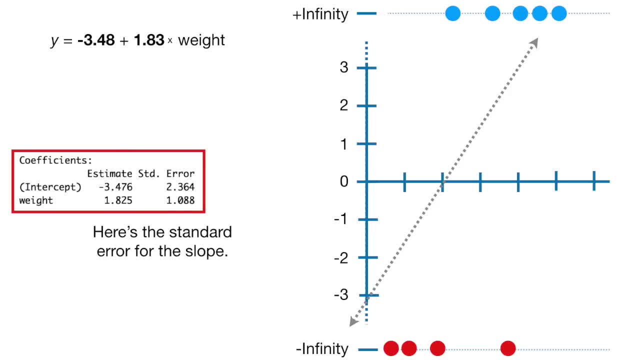 by 1.825.. Here's the standard error for the slope. Again, The Z value is the number of standard deviations away from 0 on the standard normal curve. Here's the standard error for the slope. Again, The Z value is the number of standard deviations away from 0 on the standard normal curve. 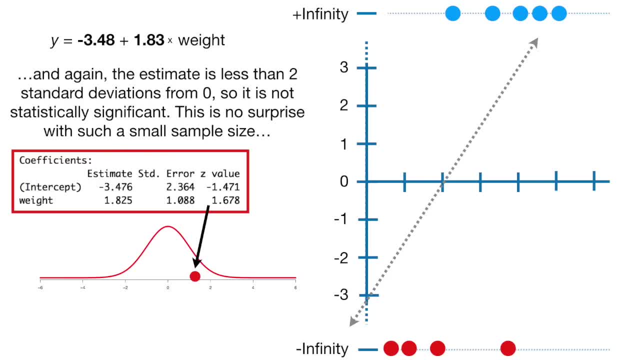 The Z value is the number of standard deviations away from 0 on the standard normal curve. Here's the standard error for the slope. Again, The Z value is the number of standard deviations away from 0 on the standard normal curve. And again: 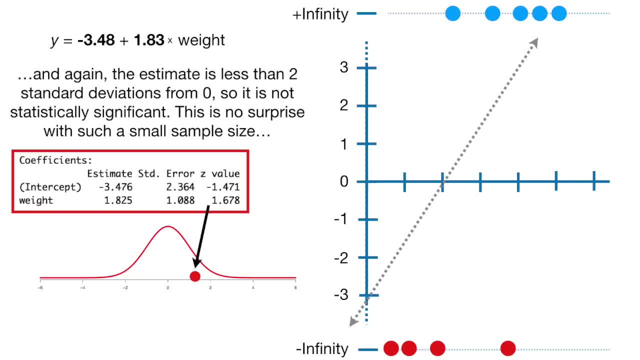 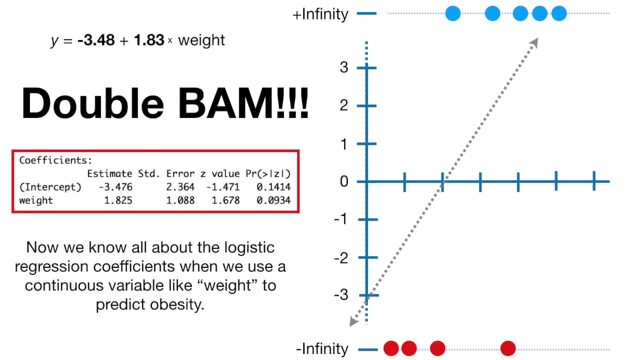 The estimate is less than 2 standard deviations from 0, so it is not statistically significant. This is no surprise with such a small sample size, And this is confirmed with the large p-value Double Bam. Now we know all about the Logistic Regression Coefficients when we use a continuous variable. 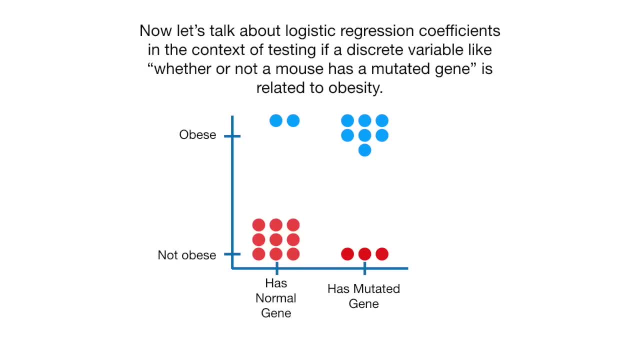 like weight to produce the Z value: obesity. Now let's talk about logistic regression coefficients in the context of testing if a discrete variable, like whether or not a mouse has a mutated gene, is related to obesity. On the left side we have mice that have a normal. 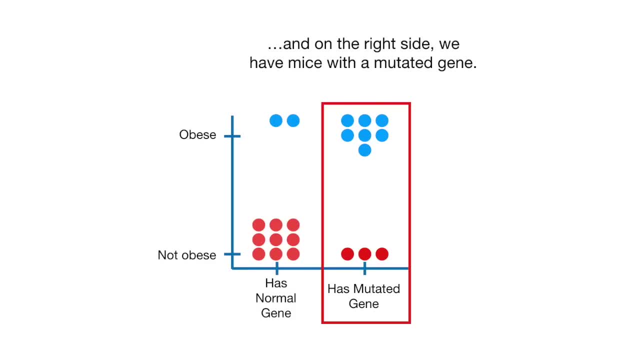 gene, and on the right side we have mice with a mutated gene. Just like before, some of the mice are obese and some of the mice are not obese. This type of logistic regression is very similar to how a t-test is done using linear models. 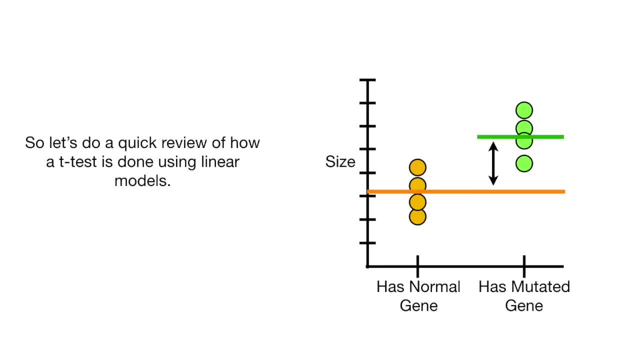 So let's do a quick review of how a t-test is done using linear models- Shameless self-promotion. If you're not already familiar with how a t-test can be performed using a linear model, then check out the StatQuest Linear Models, Part 2, t-tests and ANOVA. 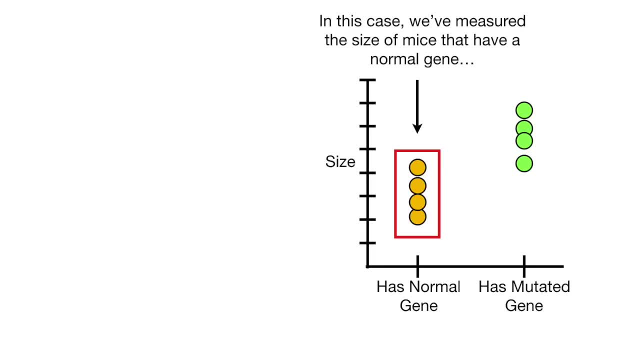 Okay, we start with some data. In this case we've measured the size of mice that have a normal gene and the size of mice with a mutated version of that gene. Then we fit two lines to the data. The first line represents the mean size for. 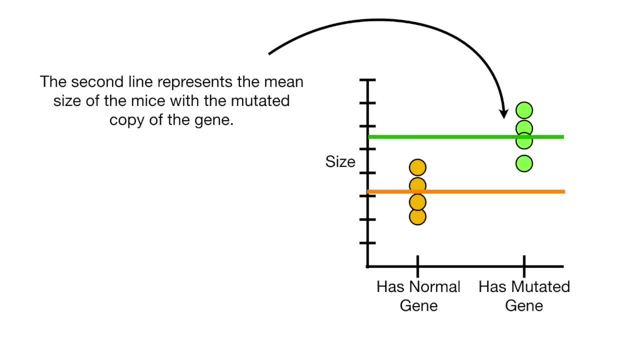 the mice with the normal copy of the gene. The second line represents the mean size of the mice with the mutated copy of the gene. These two lines come together to form the coefficients in this equation. The mean value for size for the mice with the normal copy of the gene goes here, And the difference 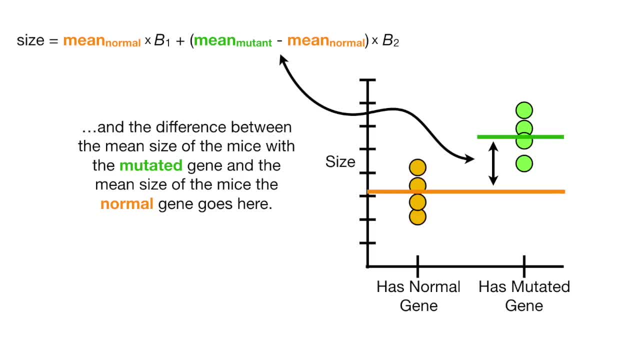 between the mean size of the mice with the mutated gene and the mean size of the mice with the normal gene goes here. We then pair this equation with a design matrix to predict the size of amounts given by the grassroots and by the that it has the normal or mutated version of the gene. This is the design. 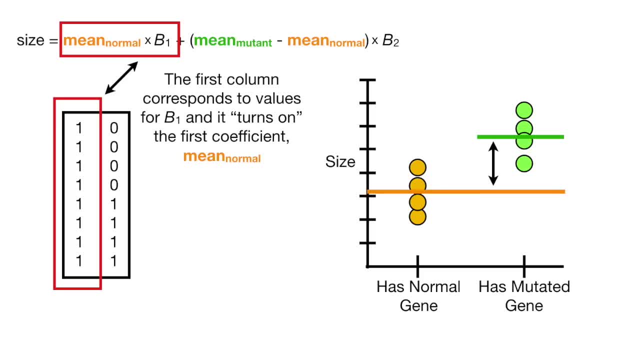 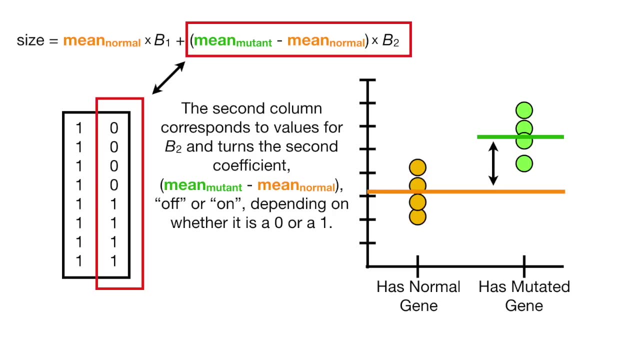 matrix for the observed data. The first column corresponds to values for B1 and it turns on the first coefficient, the mean of the normal mice. The second column corresponds to values for B2 and turns the second coefficient, the mean of the mutant mice minus the mean of the normal mice, off or on, depending on. 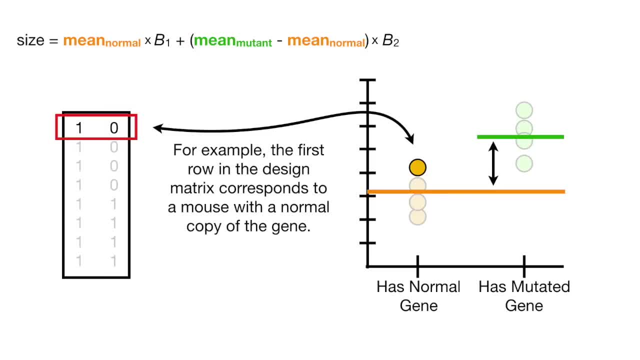 whether it is a 0 or a 1.. For example, the first row in the design matrix corresponds to a mouse with a normal copy of the gene. We predict its size by replacing B1 with 1 and replacing B2 with 0. And then we just do the math and 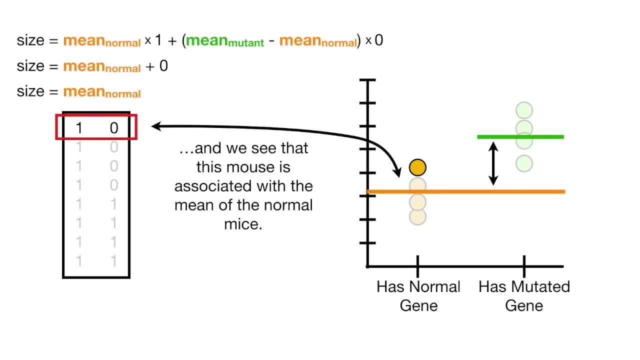 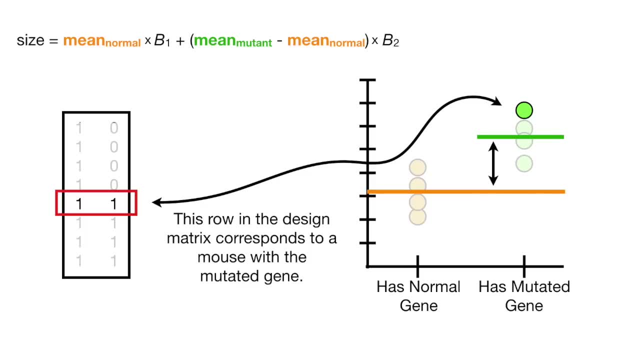 we see that this mouse is associated with the mean of the normal mice. This row in the design matrix corresponds to a mouse with the mutated gene. We plug in 1 for B1 and plug in 1 for B2 and we see that the mean of the 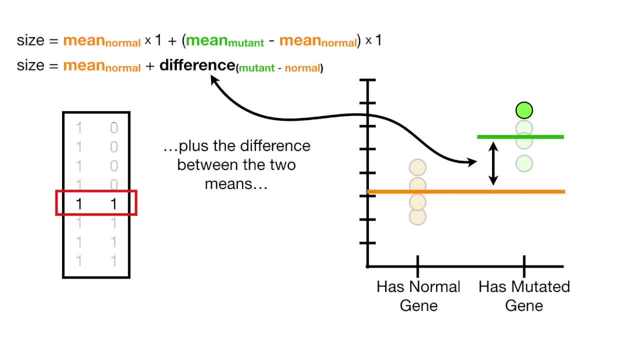 mice with the normal gene, plus the difference between the two means associates this mouse with the mean for the mice with the mutated gene When we do a t-test. this way, we are basically able to determine the difference between the mutated gene and the mouse with the mutated gene When we do a t-test. this way, we are basically 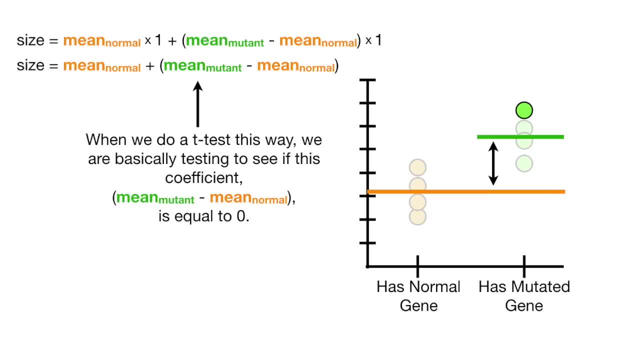 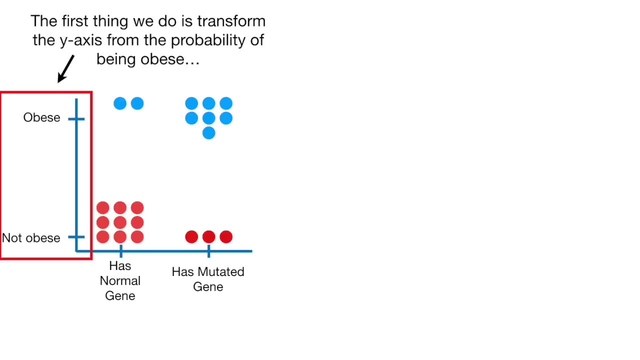 testing to see if this coefficient- the mean of the mutant mice minus the mean of the normal mice, is equal to 0.. But you already know all this t-test stuff. What you really want to know is how it applies to logistic regression. The first. 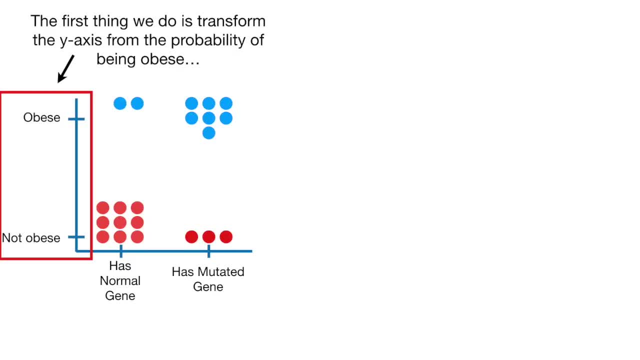 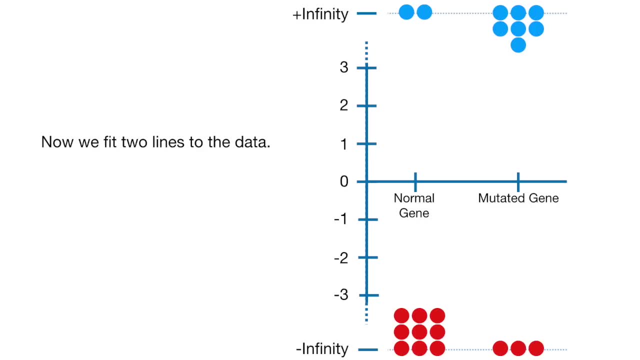 thing we do is transform the y-axis from the probability of being obese to the log of the odds of obesity. Now we fit two lines to the data. For the first line, we take the normal gene data and use it to calculate the log of the odds of obesity for mice with the normal gene. Thus the first line. 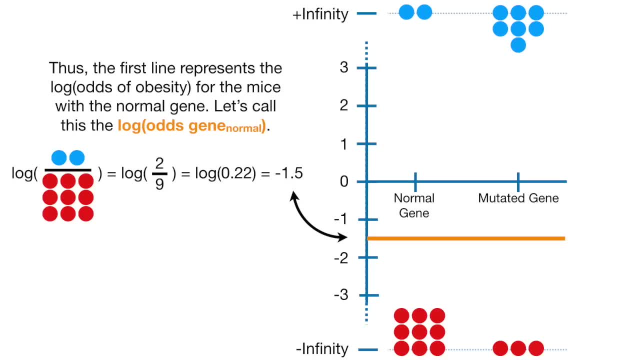 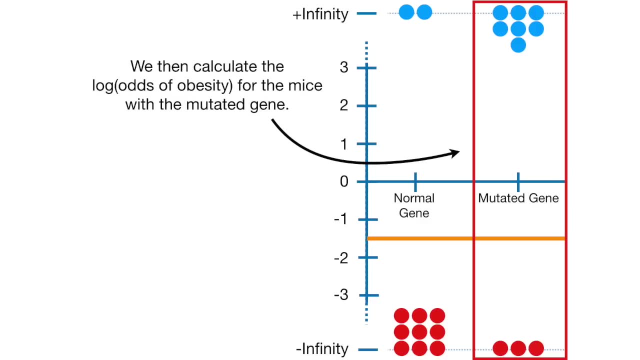 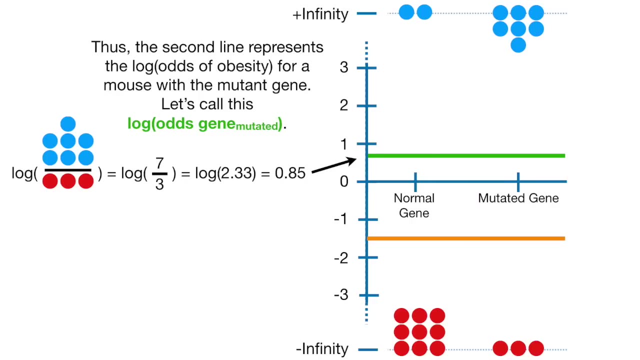 represents the log of the odds of obesity for the mice with the normal gene. Let's call this the log of the odds for gene normal. We then calculate the log of the odds of obesity for the mice with the mutated gene. Thus, the second line represents the log of the odds of obesity for a mouse with. 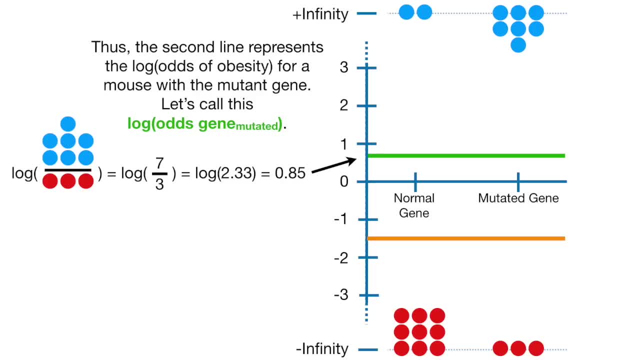 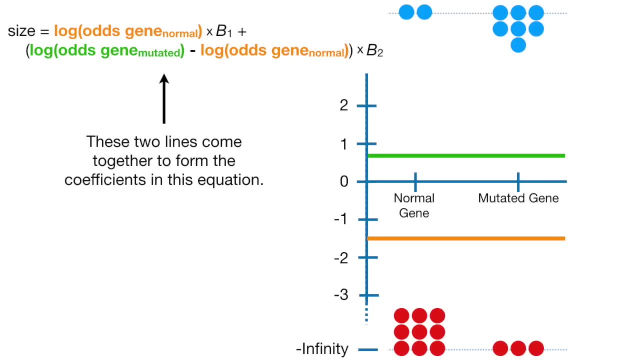 the mutant gene. Let's call this the log of the odds gene mutated. These two lines come together to form the coefficients in this equation. The log of the odds gene normal goes here, And the difference between the log of the odds gene mutated and the log of. 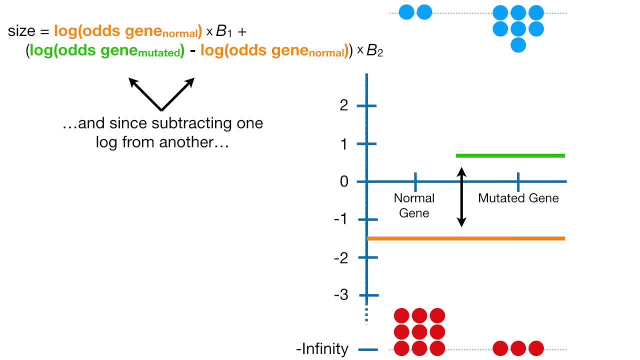 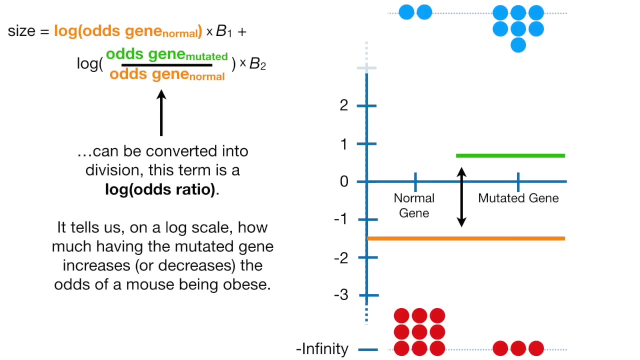 the odds gene normal goes here, And since subtracting one log from another can be converted into division, this term is a log of the odds ratio. It tells us on a log scale how much having the mutated gene increases or decreases the odds of a mouse being 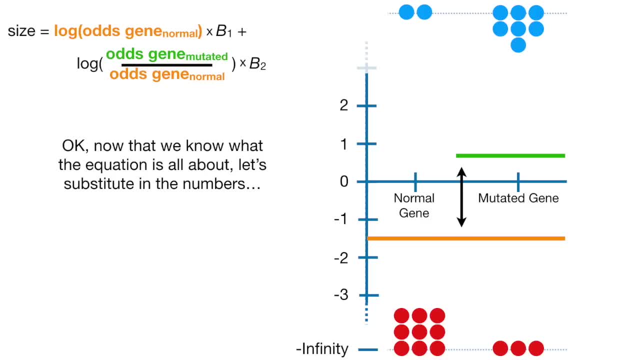 obese. Okay, now that we know what the equation is all about, let's substitute in the numbers. The log of the odds for gene normal is just the log of 2 divided by 9.. And the log of the odds for gene mutated is just the log of 7 divided by 3.. 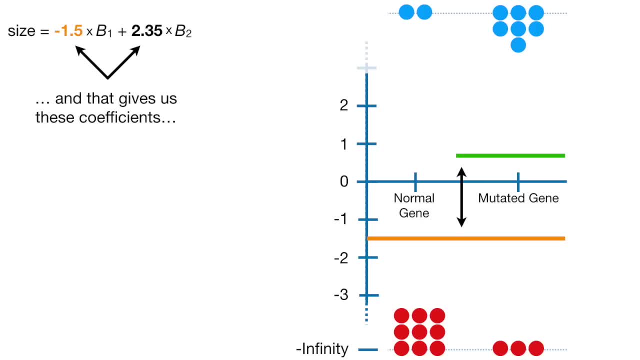 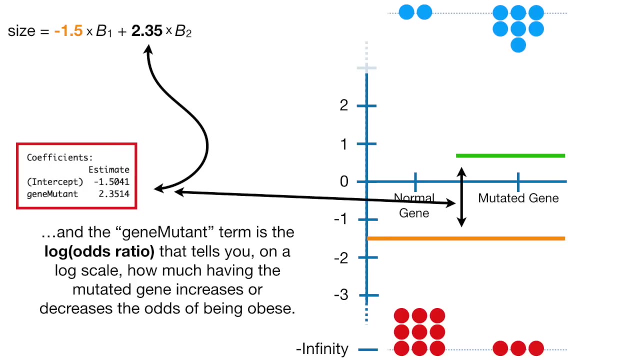 Now we just do the math And that gives us these coefficients And those are what you get when you do logistic regression. The intercept is the log of the odds for gene normal And the gene mutant term is the log of the odds ratio that tells you. 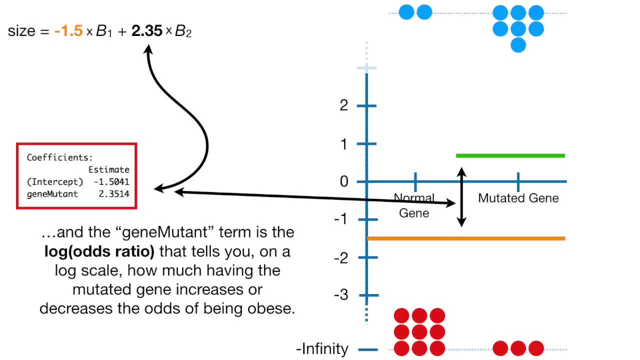 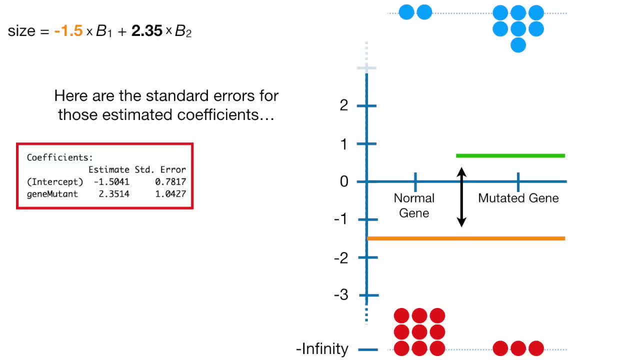 on a log scale how much having the mutated gene increases or decreases the odds of being obese. And here are the standard errors for those estimated coefficients. And here are the Z values, aka the Wald's test values that tell you how many standard deviations the estimated coefficients are away from 0. 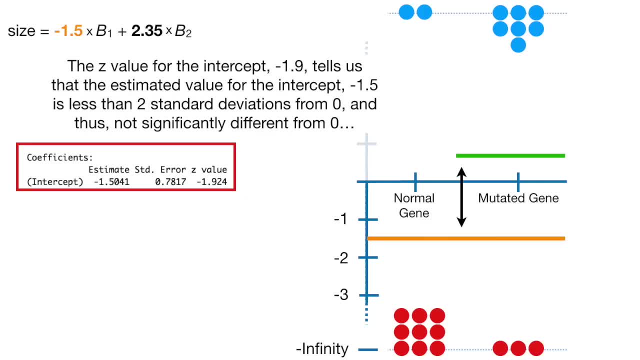 on a standard normal curve, The Z value for the intercept tells us that the estimated value for the intercept is less than two standard deviations from zero, and thus not significantly different from zero, And this is confirmed by a p-value greater than 0.05.